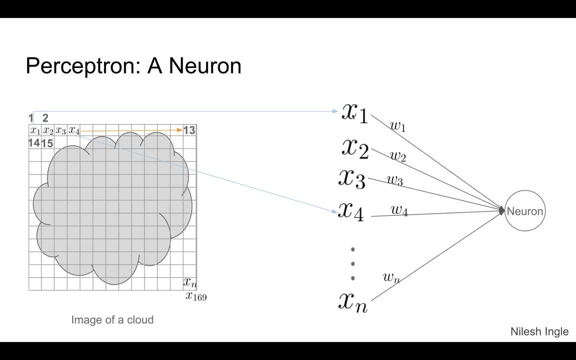 So the gray value of, or the value of each of those pixels is multiplied by the weight, and that's the input to the neuron, And that is done for the entire image set. So if, In this case, we have a total of 169 pixels, and all those would be the features in that particular data, features for this particular neuron. 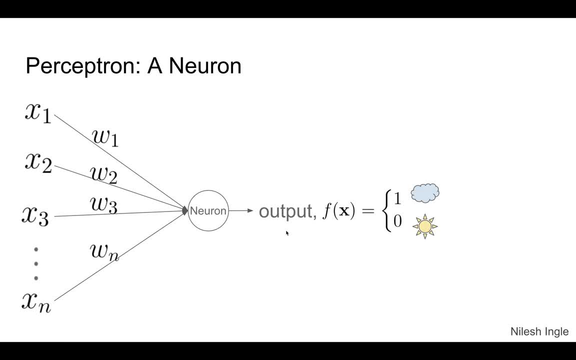 Now the neuron computes an output value which is then classified based on the score. So let's look at this slide here. If the score, which is WX plus B, where B is a constant here, if that is greater than zero, then that particular class then it is. then that image is assigned to class one, which is clouds, that it will rain, and otherwise it's assigned to class zero, which is sunny and it won't rain. 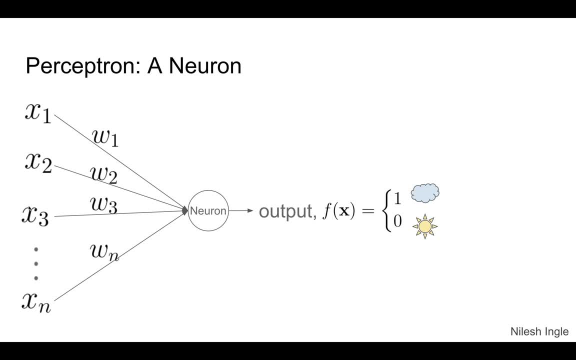 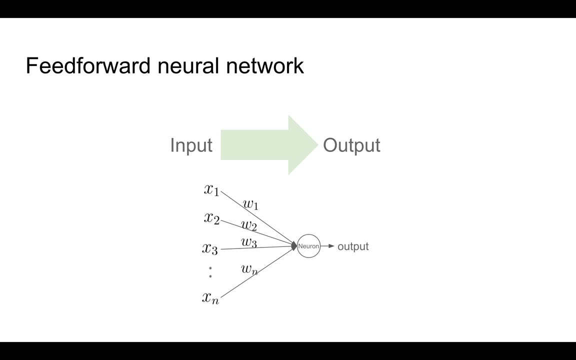 So, basically, we can go from an image using a neuron or perceptron To classify that image to either a positive class or a negative class, And in doing so, what this is an example of is a feed forward neural network, a very simple one. 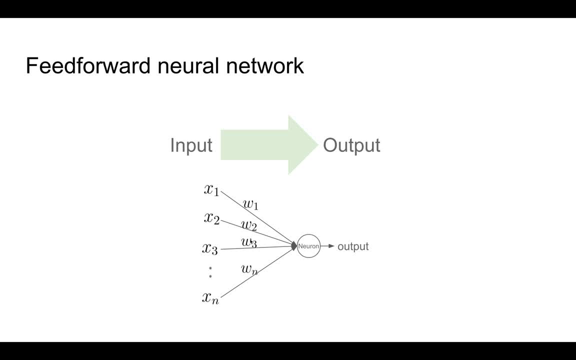 What a feed forward indicates here is that there is no feedback loop from the point after the neuron to update the weights. So it's that, So it's that. So that would be the backward propagation which does not happen here. So this: the information flows only in one direction and that's a forward direction. 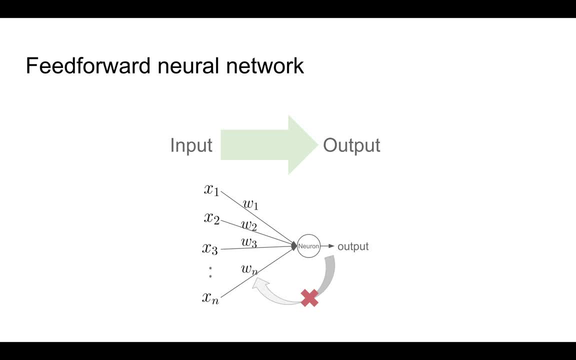 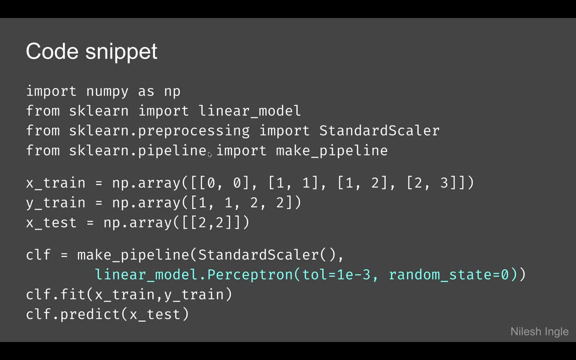 So that's the takeaway message from this slide. In the code snippet we have seen. this is similar to what we have been seeing here. We are importing NumPy linear model and then standard scalar MIG pipeline And to this This train and test data set. we first pass it through the standard scalar in the pipeline and then fit the model using linear model, dot perceptron as shown here. 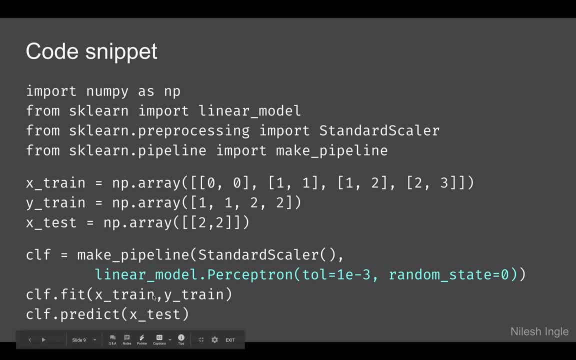 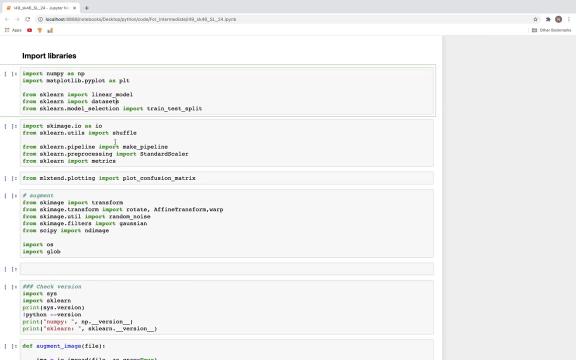 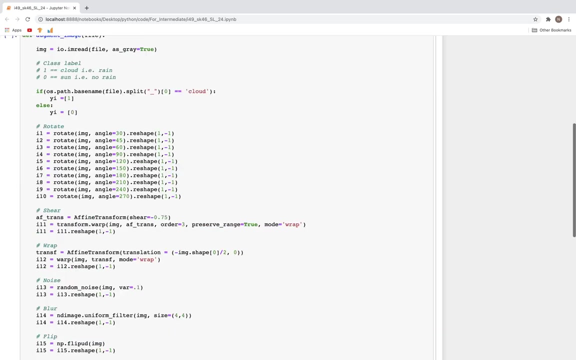 And this is fit on the X train, Y train, and then finally use the CLF dot predict to predict on the test set. Now let's get into Jupyter notebook and look at the code. So these are the libraries That I have imported. there are several libraries here and this is the version that I'm using. 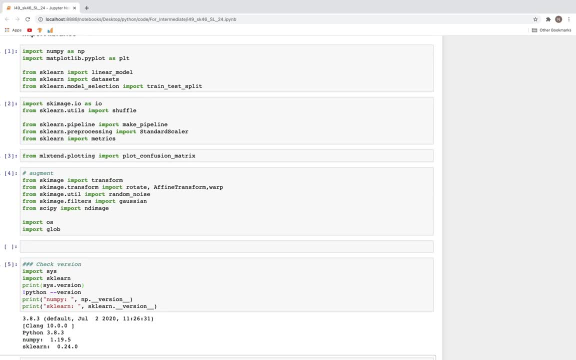 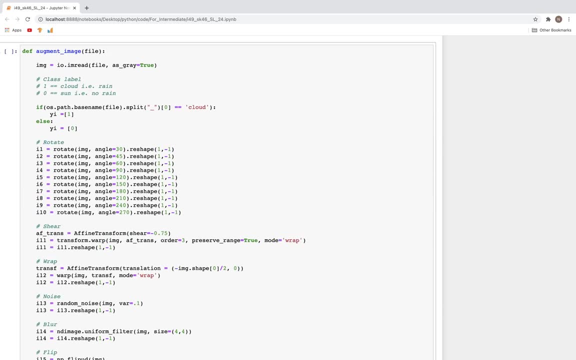 You may have to pause the video to note which of these libraries are used and these are the versions. Now for the augmentation step in this data set. in this video, the data set that we are going to use is a data set with two types of images. 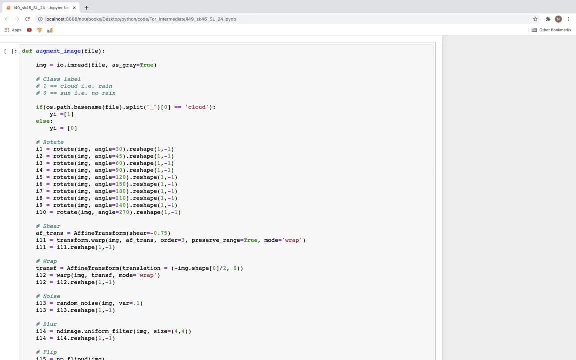 Clouds and sun have handmade this data set and uploaded it on GitHub, and I'll post the link below in the description so you can download it. Additionally, this is the function that we have discussed in the previous video for image augmentation. It's the exact same function. 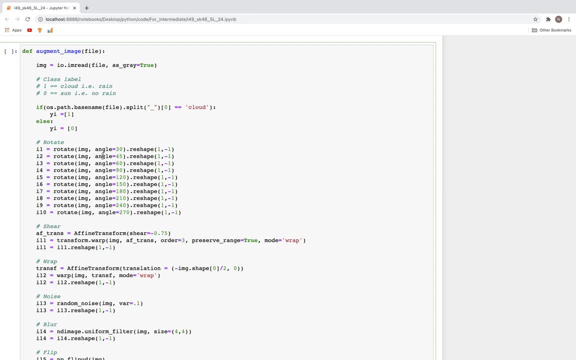 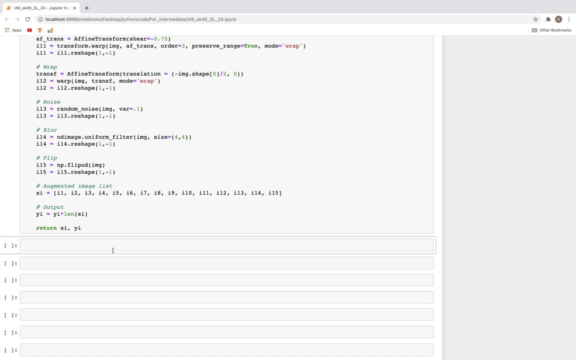 I also put a link in the description for this function, so you don't have to type it with. with this set, We can now go ahead And Perform the fit, first on the data that is not augmented and then on the data that is augmented. 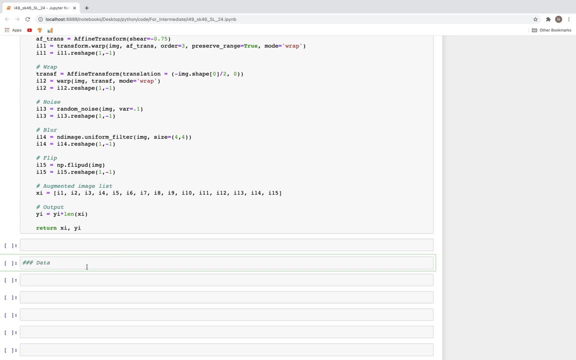 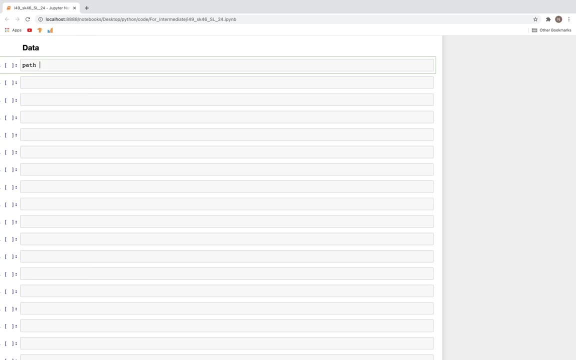 So let's look at the data first, And here, because I've already downloaded the data, it's at the path which would, which would be different on your computer based on where you have saved it. I've saved it on the desktop, So 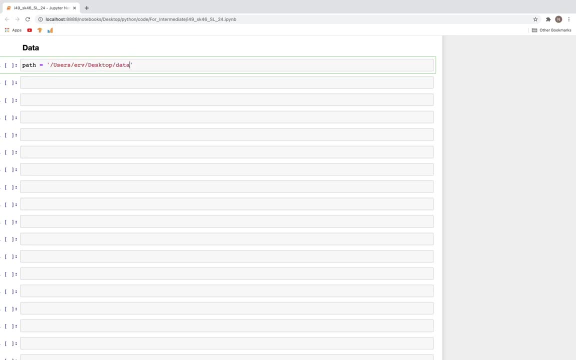 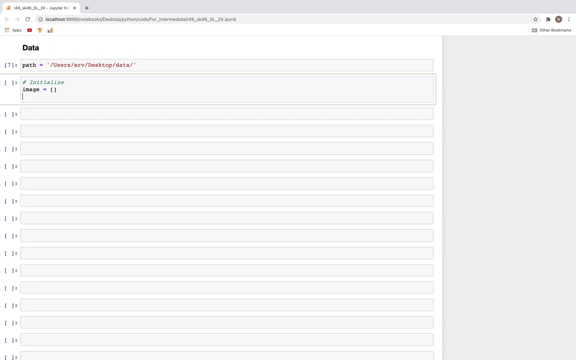 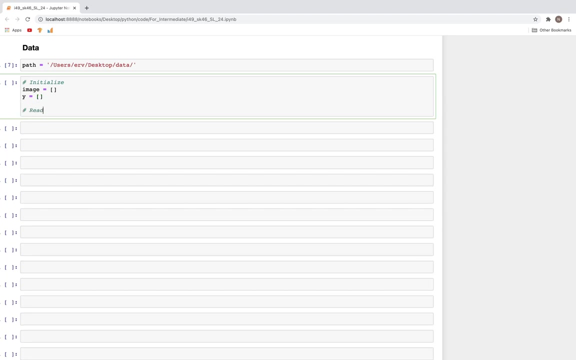 This is the path that I'm navigating to now with this, the. what I'm going to do now is initialize. initialize the. initializing a list for images, then initializing a list for the output labels Y and then using a for loop to read the images. 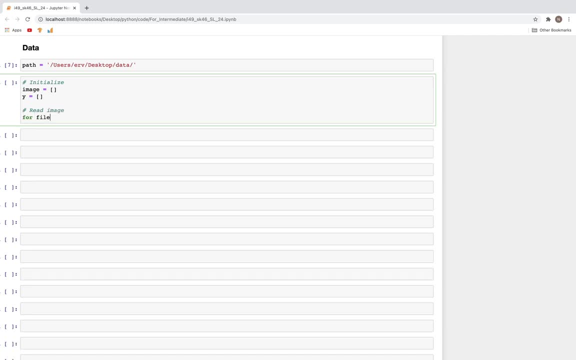 So you're reading all the images from the folder that I've loaded So. So This is the path that I'm going to download. So file in OS dot list dir path. There are different ways to read it, So this is using the OS dot list dir. 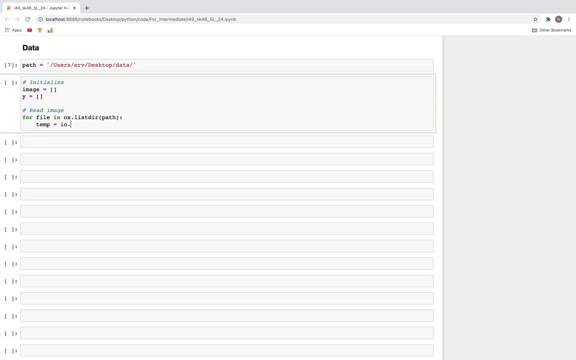 And I'm going to read each image: save it in the temp folder. So temp variable. So IO, dot. IAM read OS, dot. path, dot. join. And then this is going to join the path and file name And I'm going to, I'm going to read it as gray image: 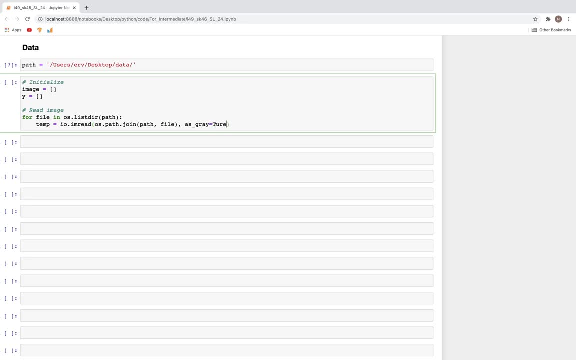 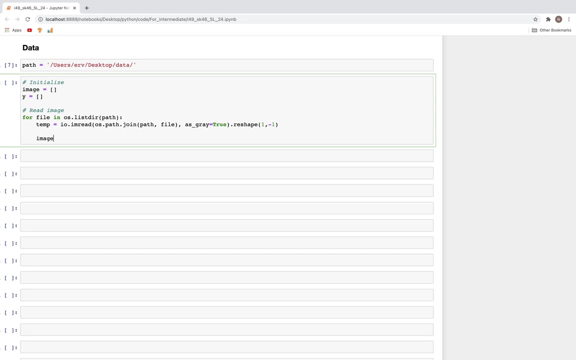 As gray is equal to true, True Can spell true, And then this needs to be reshaped, So I'm going to reshape it to one and minus one. Once this is read this, I'm going to append this image to the empty initialized folder. image above: 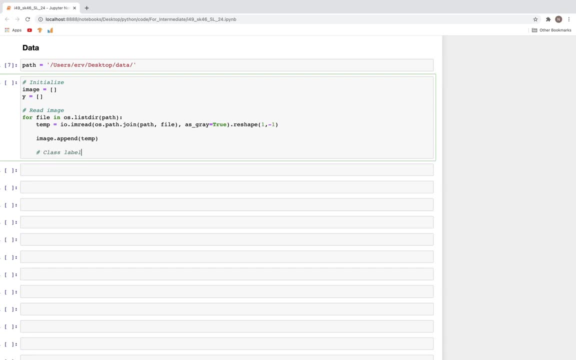 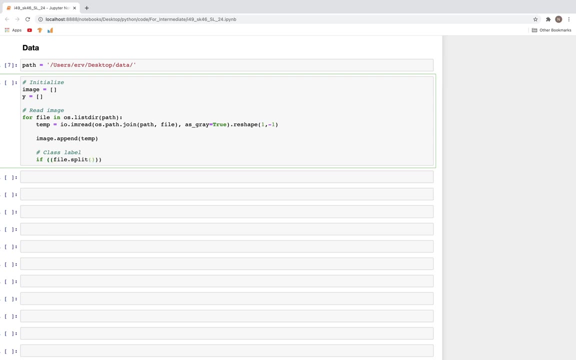 And Finally add the class label. So the class label is based on the file name. If the file dot split, So the file has the string of the file name is split using the underscore. And then, if you take the first part of that, 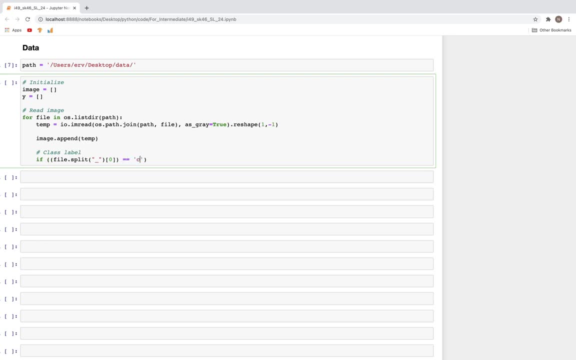 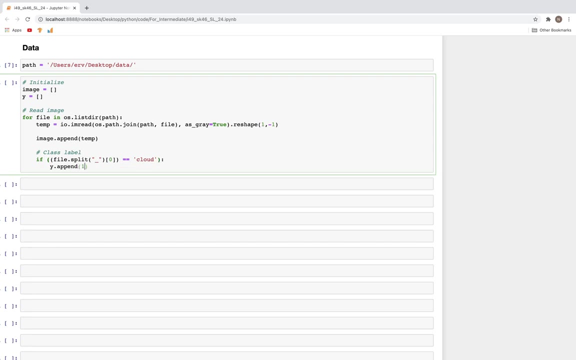 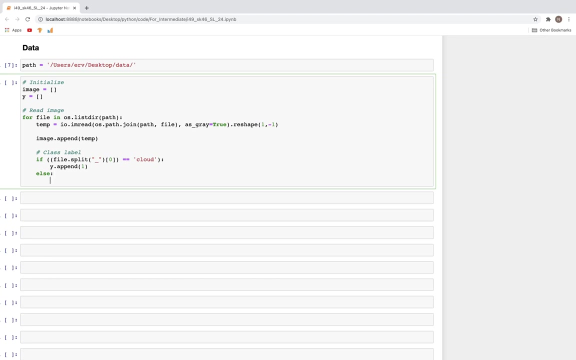 If that is equal to cloud, then it is. you're appending one Because it will rain, So the label is rain and therefore we have the label. as one else, We are going to append zero, suggesting that it's not going to run, So the image would be of sun. 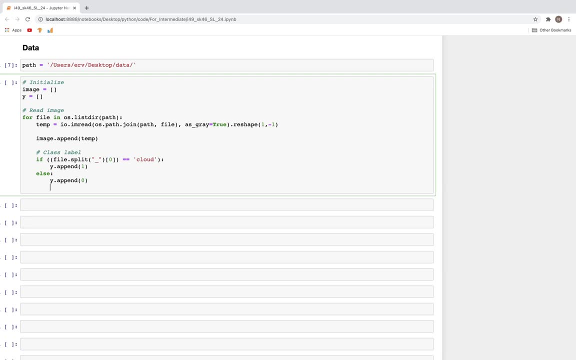 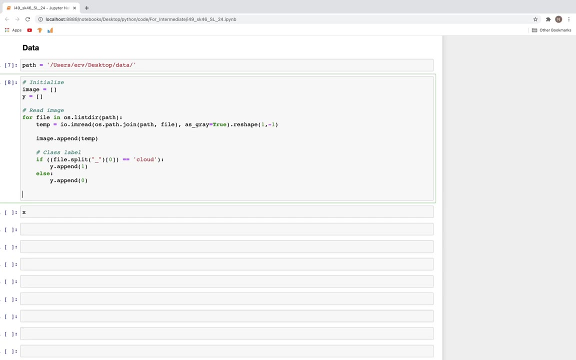 And once that is done, So let's run that. And now we can put that in the same cell. X is equal to NP, dot concatenate- And here this is image images- That the image and access is equal to zero. So what I'm doing here is concatenating all the arrays that we have in the list image. 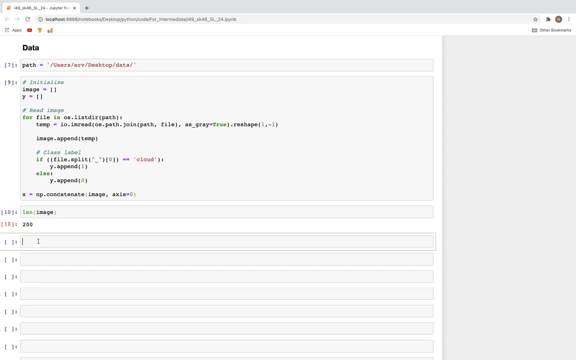 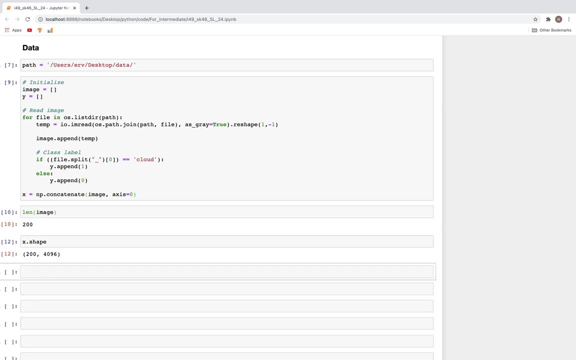 So if you have, this is there are 200 of them. So, if you look at this, these are different arrays And now, After concatenating, we have this as the shape of the array. So there are 200 rows and 4096 columns. 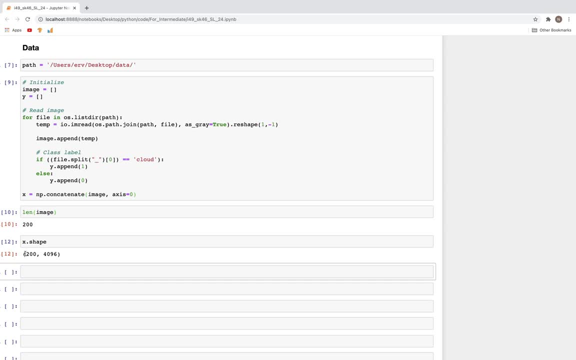 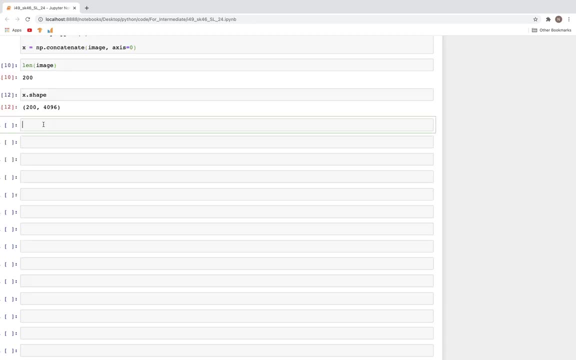 Each column is one pixel, So entire image is flattened out as one row in this particular case. Now let's visualize this. So visualize, And for visualization, I'm going to print this print. So we do this. Now, look at the top right. 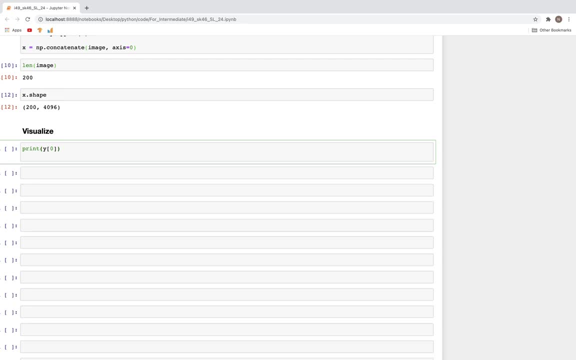 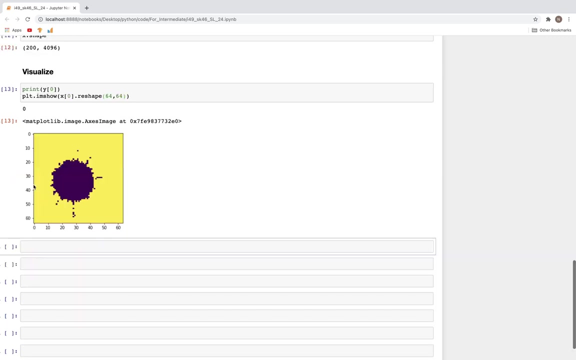 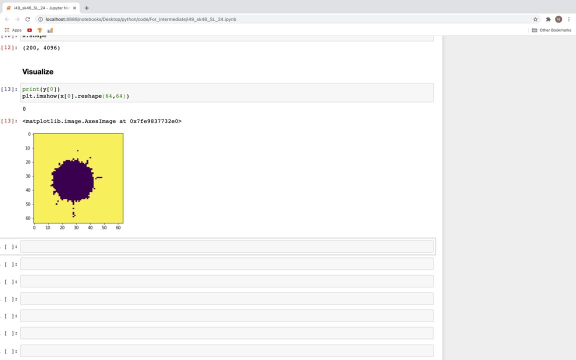 And this window on the left is the image that you can see there And the image of this person looks like a green screen And this image is in the black space And as the image turns green, And now find your image. So, in case of sure, 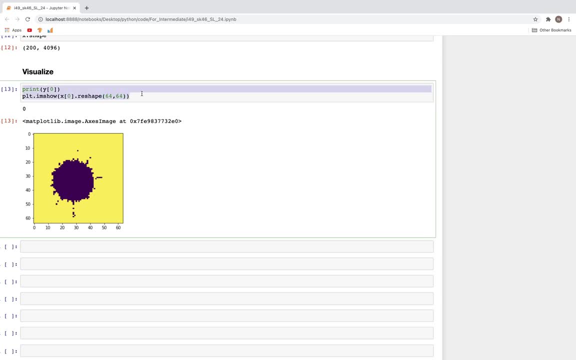 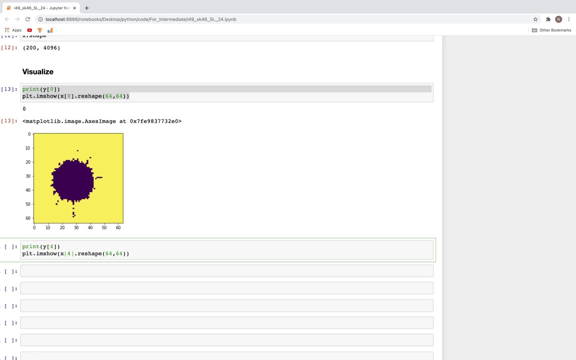 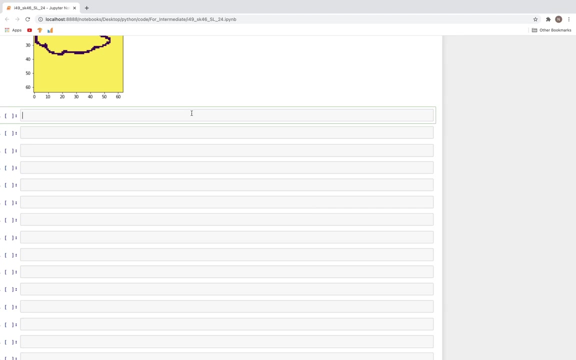 So this is the image that we need to speed up the typing. and now let's look at four. so four is image of a cloud, and next we are going to do a shuffle, split on the train, on the data set that we have. so shuffle and split, and what that will do is we'll get the x train and y train. 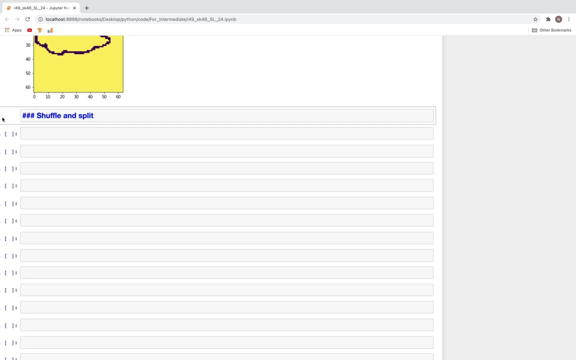 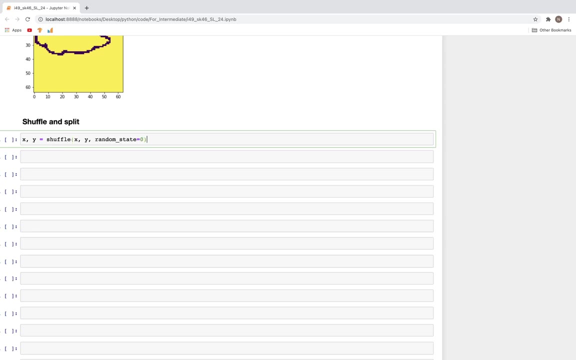 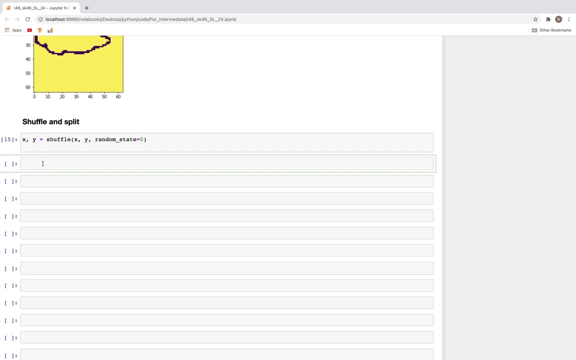 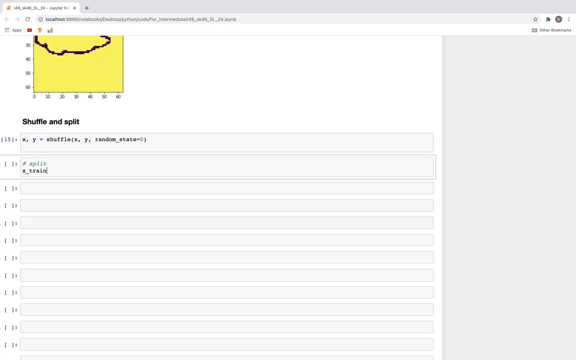 so x- y is equal to shuffle x- y random underscore state is equal to zero and that is important so that we don't have the sun images lined up and cloud images lined up when we are doing the split. so for split we have x underscore, train x underscore, test y underscore, train y underscore. 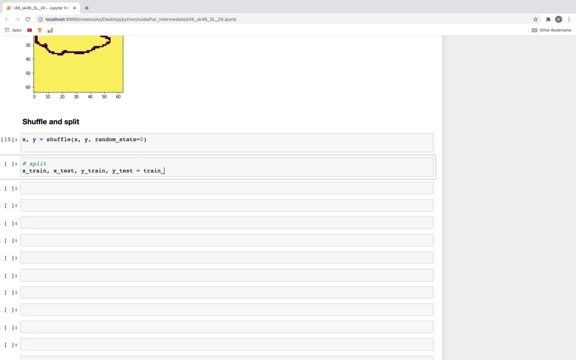 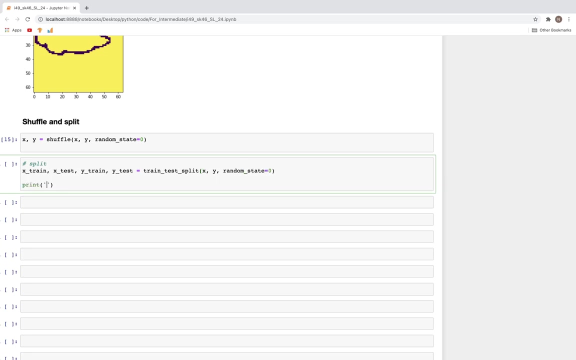 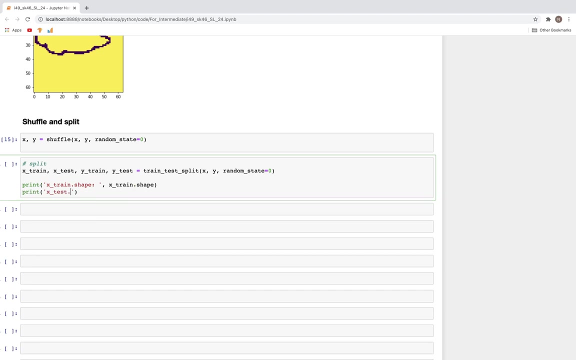 test is equal to train underscore, test underscore split. and then we have x, comma, y and again random underscore state is equal to zero. so here we can go ahead and print x underscore train dot shape so we know how many records we have in the train data set and then we can print x underscore test dot shape and that that will. 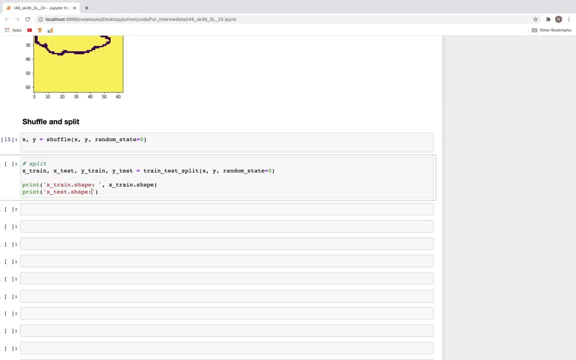 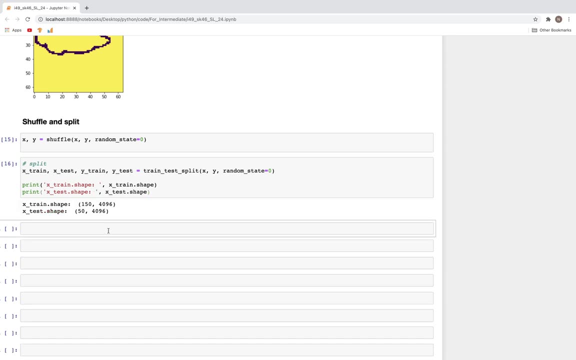 tell us how many records we have in the test data set. so we have around 150 records or 150 rows. now let's go ahead and fit the perceptrons. so we'll do that using perceptron, and this is now so far. we haven't used the augmented data, so for this we need to normalize. so 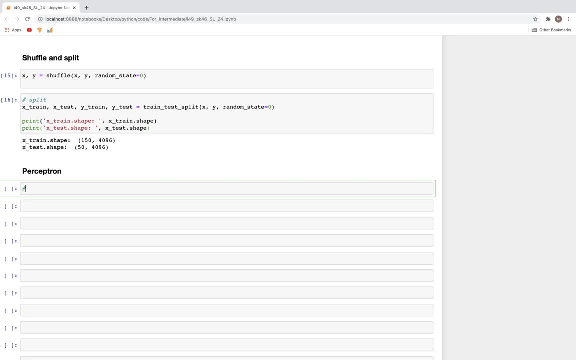 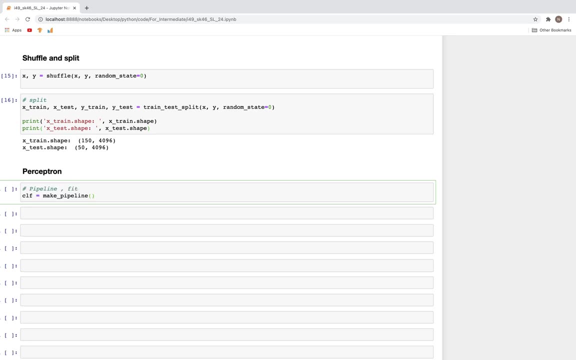 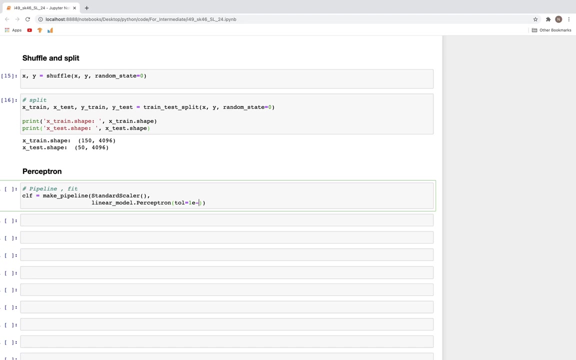 we'll start with pipeline and then use the fit. so clf is equal to make underscore pipe pipeline, and here we'll use standard scalar. and then we have linear underscore model, dot, perceptron, and we'll use tolerance of 1e to the power minus 3. random underscore state is equal to zero. 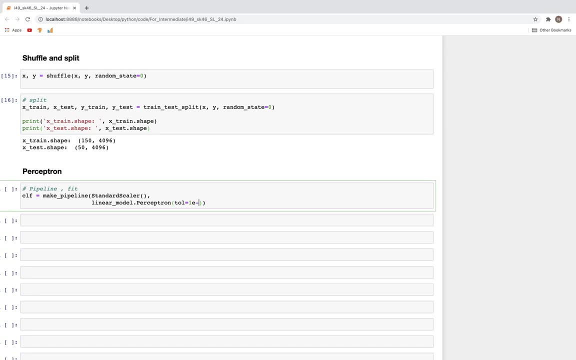 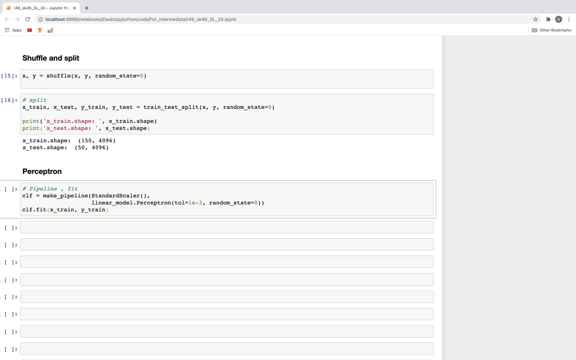 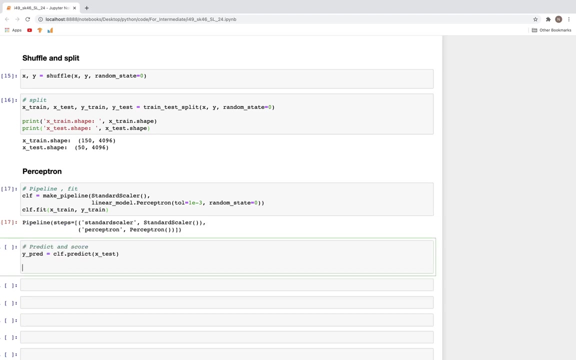 and then use clf dot fit x underscore train, y underscore train and so that's the train part. then we can predict, predict and score. so those two parts. so y underscore pred is equal to clf dot predict, x underscore test. so we predict based on the test set and then you can get the accuracy matrix dot accuracy underscore. 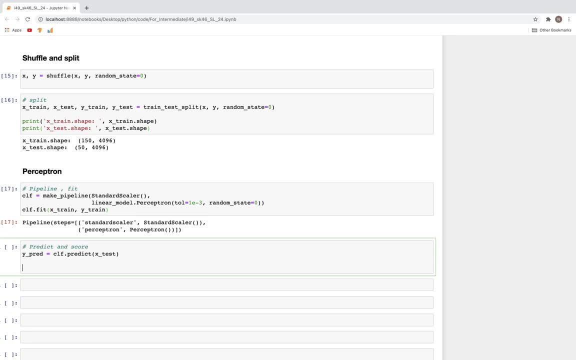 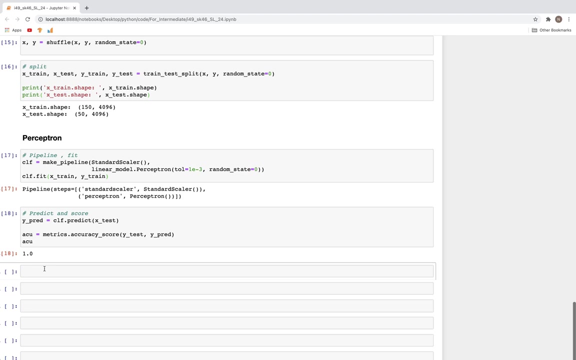 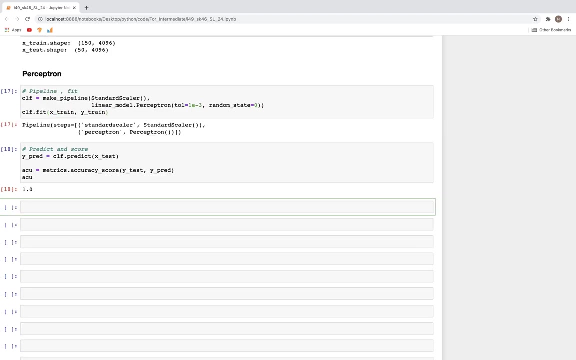 score y underscore test, and then the y underscore pred, and then we have the accuracy. so we are getting one as accuracy and that's uh, we won't. it's difficult to get a complete accuracy, but maybe just for this example we are getting, we got lucky to get a hundred percent correct predictions, so we can also get. 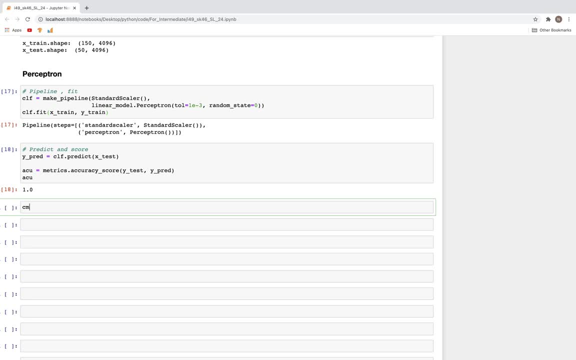 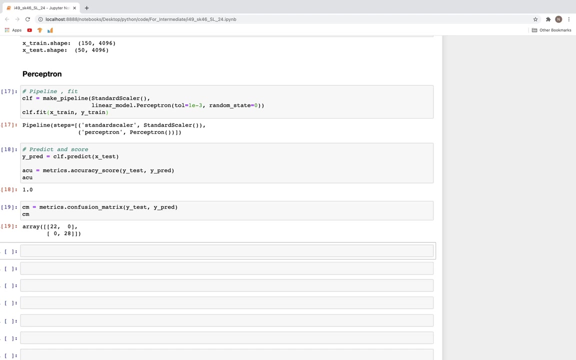 the confusion matrix. so matrix dot, confusion, underscore matrix. and here we can specify test y, underscore pred, and we can see that 22 out of 22 are correct and all. so the diagonal of diagonals are zero. it means the all the predictions are uh accurate, uh, now let's look at using the augmented data. 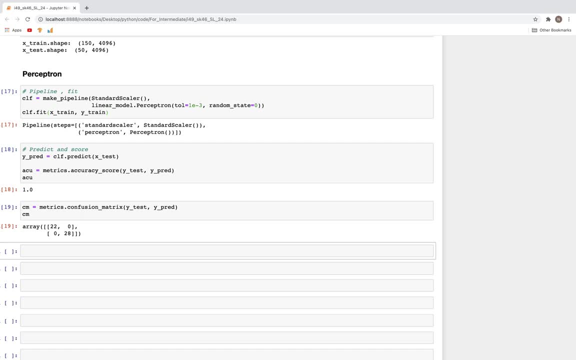 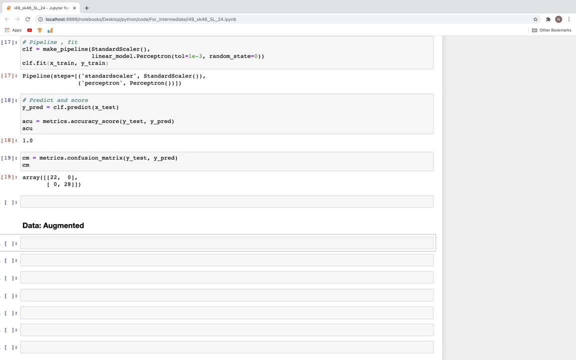 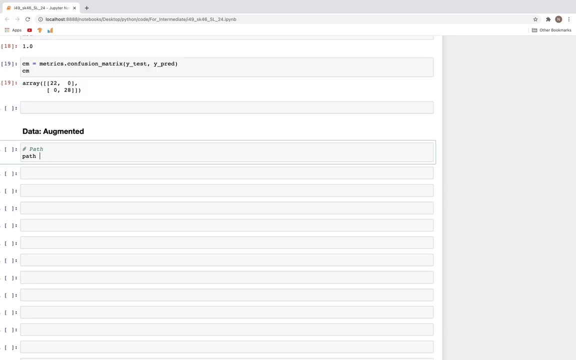 and see how that works. so for augmented data, we already have created the function, so we i won't be going through that function how it works. basically it just creates 15 images from one image. now to use that function, we first need to set the path, so path is equal to users that will this. 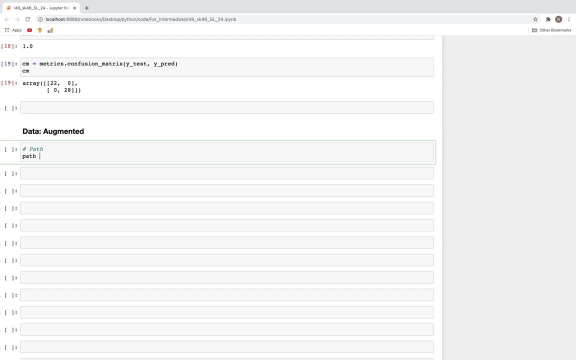 would be the path to the directory where that image is right, where those images are stored: the original images, desktop, and then data, and here i'm especially installed, or png, and x, a, y. so these are the empty lists, that's i'm initializing, and then for file in globglob. so here we are going to. 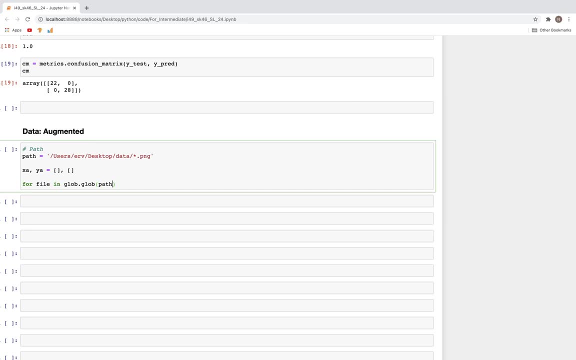 go through the directory, read each file and then put that in here after augmenting стро pmthere crochet folder換 path consists of empty list that are initialized in the desktop and then for file in oglobe top globe. so here we are: going to go through the directory, read each file and then put that in here after augmenting somos computer dengan. 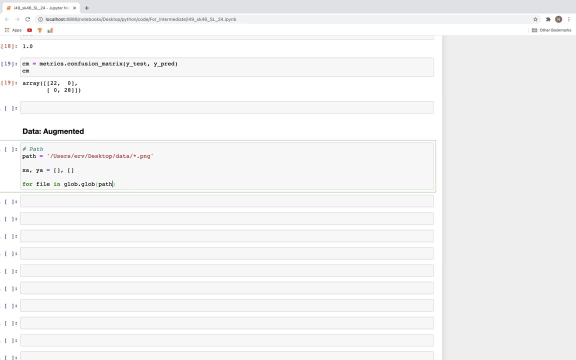 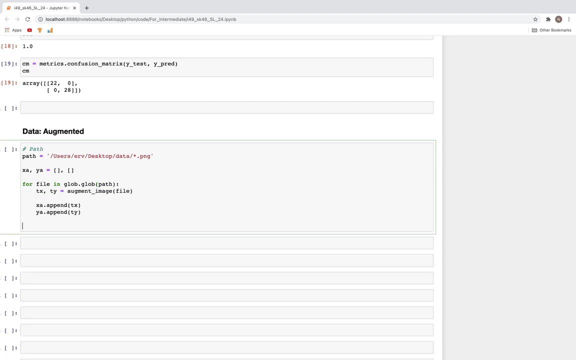 so augment image. so that's where we call that function that we have created. and then x a dot, append t x. and then y a dot, append t y. so we append the augmented values and then we flatten the lists within the list by a list comprehension. so for j in i, what you want to do is j for i. 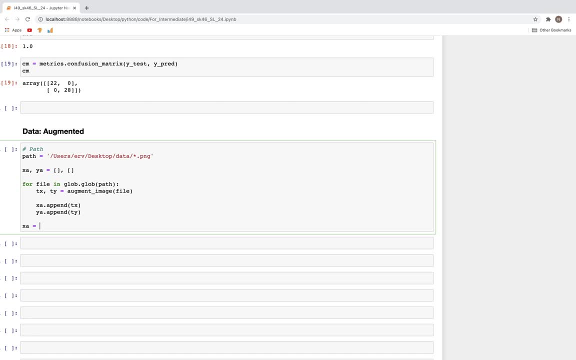 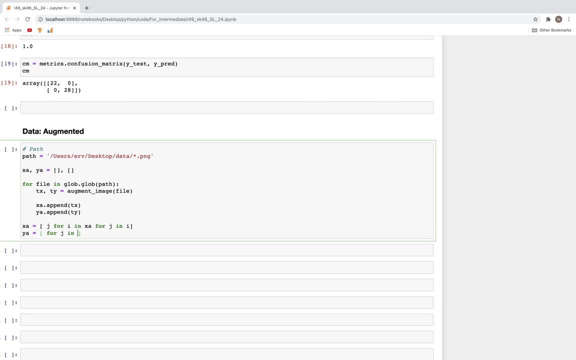 in x a and similarly we have y is equal to for j in i. this would be for j for i in y a. so we have y is equal to for j in i. so for we are. what we are doing here is, let's say, if we have a list within a list. so 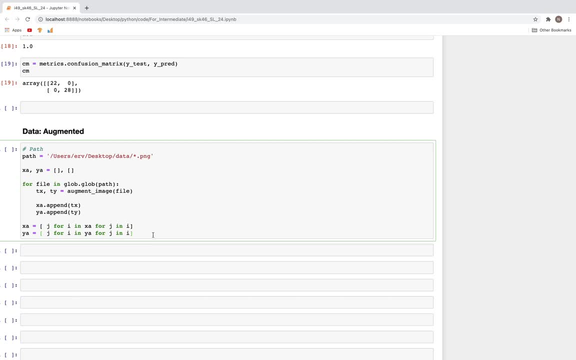 1 comma 2, and then we have another list: 4 comma 5. so we are flattening this and converting this to 1 comma 1, 1 comma 2 comma 3- sorry. 4 comma 5. so that that's what we are doing here with. 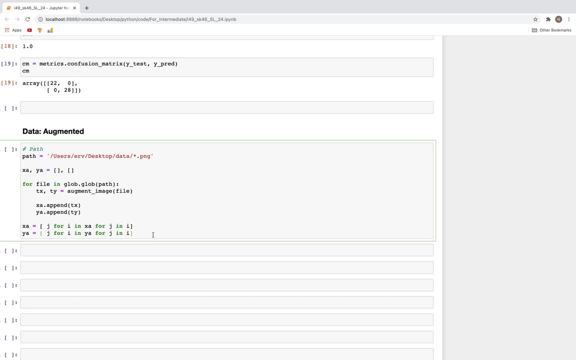 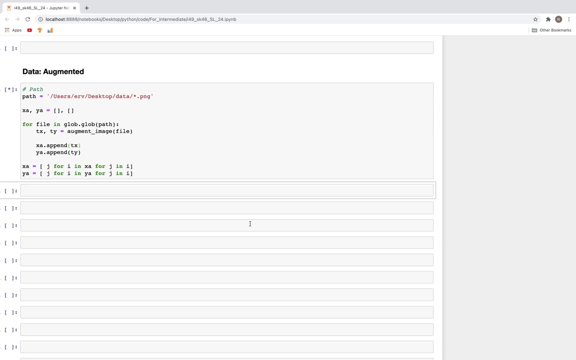 uh, when using x, x and y. now, once we have run that, uh, let's see if we get any errors. uh, if not, then we'll print the length of this, so length of xa, and then print length of y, a, and both of those lengths should be similar. so now we have. 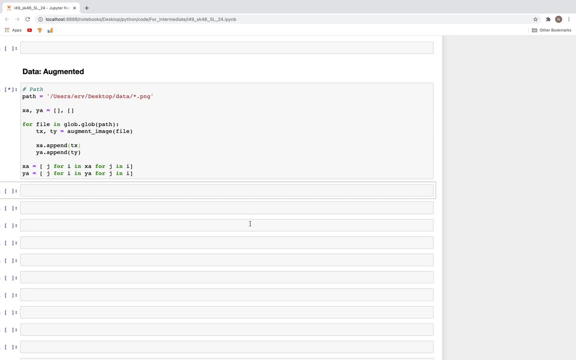 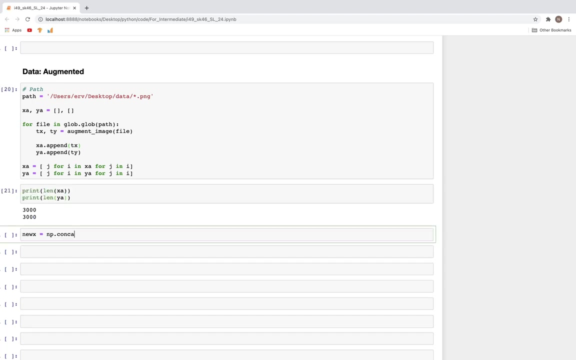 uh, 3 000, 3000 data points, additional data points and this will add the original data points. so new x that we have now will have 3200 images npconcatenate and here within a list we specify the earlier value and then concatenate. these are the new values that we have. axis is equal to zero. this could. 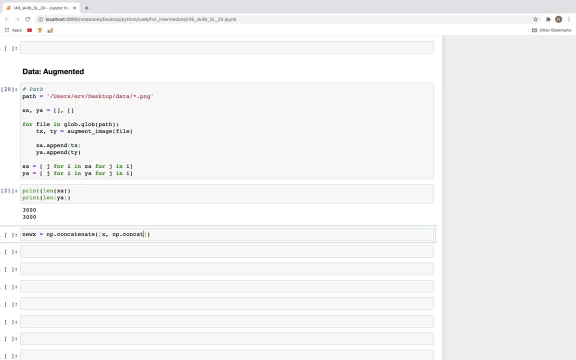 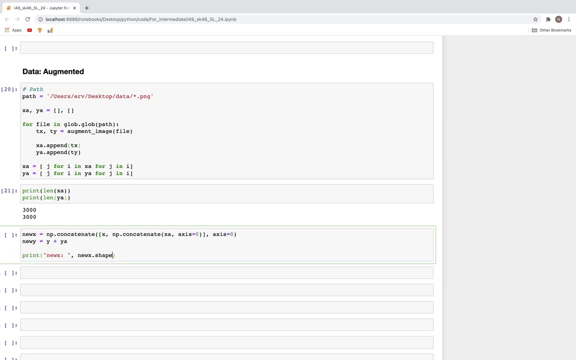 have been done in separate steps, but i'm just adding them together here. so that's the new x, and for new y we have y plus ya, and thus if we print the new x and new and the shape of new y, so shape of this, and then print new y, so this would be length, length of new y. 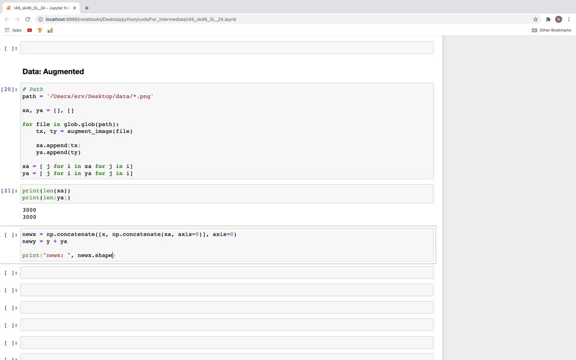 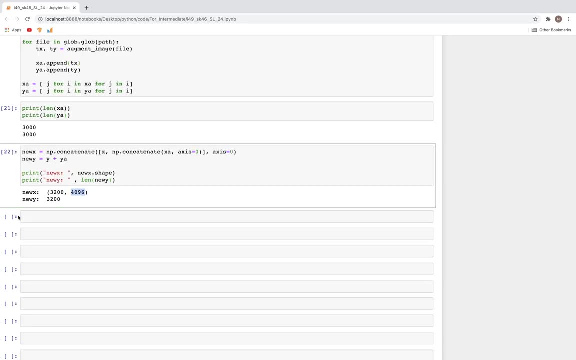 so we get: there are 32 rows, so 32 images, and each image is 64 by 64, therefore 4096. now, with this perceptron we can perform the fit. so perceptron, and here we have, first we do the shuffle. shuffle is new x, new y is equal to shuffle. 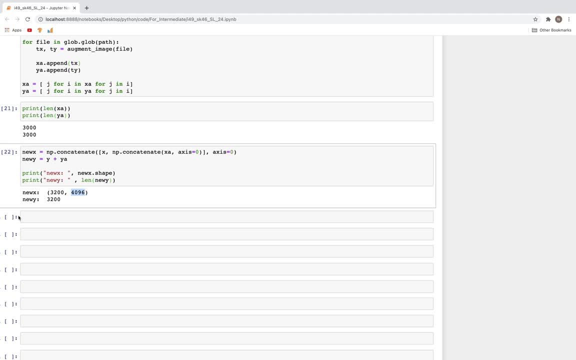 x, new, y, random underscore state is equal to zero. and then again we are going to do the split train and test. so here is split: x underscore train, x underscore test, y underscore, y underscore train, y underscore underscore test is equal to train underscore test underscore split and this is: 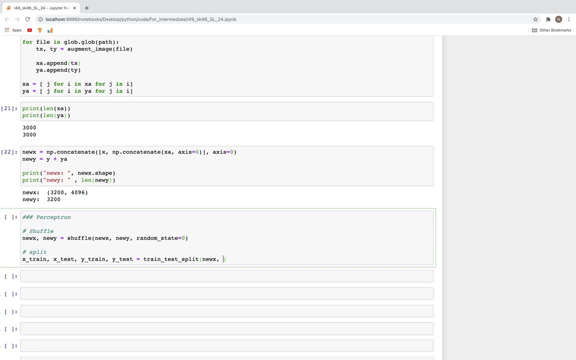 based on the new x and new y and finally we can do the fit using the pipeline. clf is equal to. let me go ahead and copy that, so we don't have to type it copy, and i'm just simply going to paste it here, because it's the exact same stuff, and then predict so for prediction: again, it's the same. 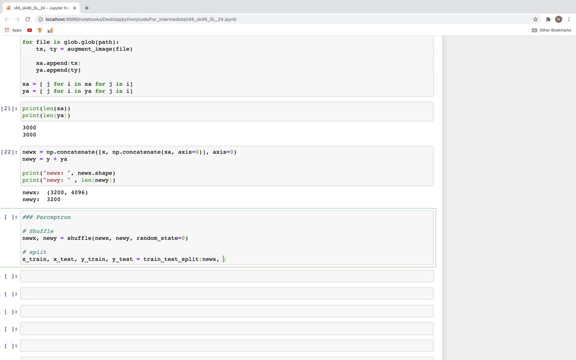 stuff. y underscore predict is equal to clf dot predict, x underscore test, and then, sorry, x underscore test, underscore test, and then we have score. so for score accuracy, so matrix r dot accuracy, underscore score, y underscore test, y underscore pred, and we can do this. so here we have the matrix r dot accuracy, or matrix 믿. then we have the model of prediction n of etmek, then we have the study, and so here we are going to 很多 of the architecture that we are attempting for. so or we even know much about the approach. so, in the case of yoga, five quarters of our topics. obviously, we know that this is a guardian of rates, so but 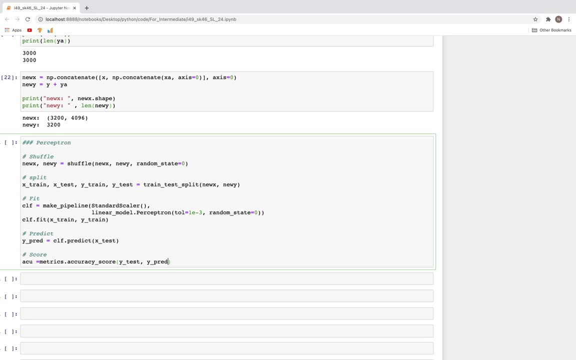 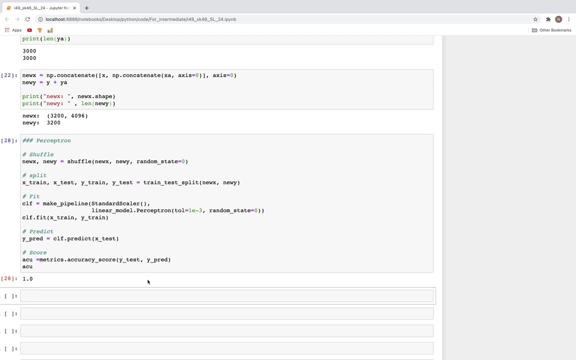 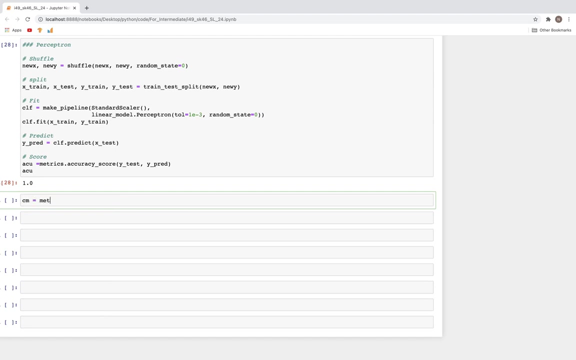 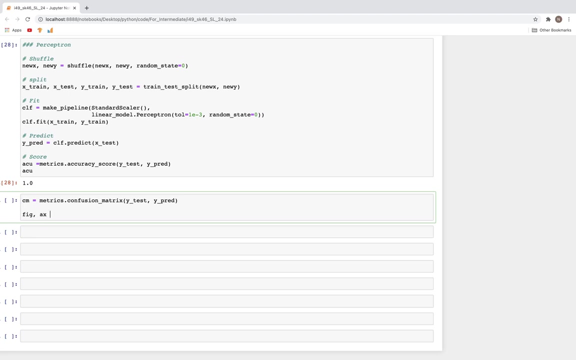 compute the accuracy here. when we run this you get accuracy of one. so this is with the augmented data. now we can get the confusion matrix. so CM is equal to matrix dot, confusion, underscore matrix y, underscore test y, underscore thread. and here will first create the matrix without any class name. so bigger X is: 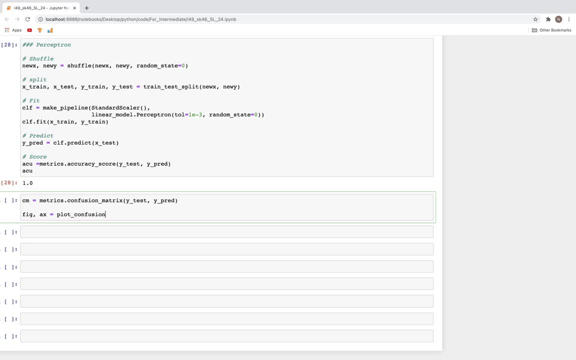 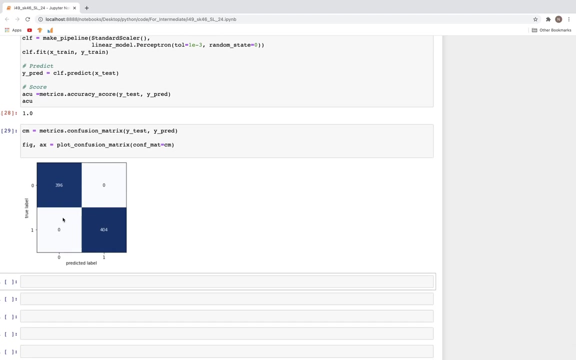 equal to plot underscore, confusion underscore matrix, and this is using the ML extend library conf. underscore math is equal to CM and when we run this, this is the confusion matrix we have. the diagonal elements are zero. now to add class names to this. if you notice, in this confusion matrix the zero zero is. 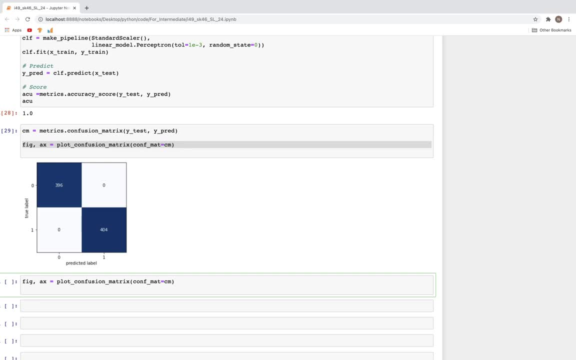 the top left corner and one one is the bottom right corner, and so we know that class names for rain and no rain, so rain is one. so therefore class names is equal to. I'm going to specify rain as so no rain would be the second one. breathe. no rain would be the first one, because we are looking at one or rain. 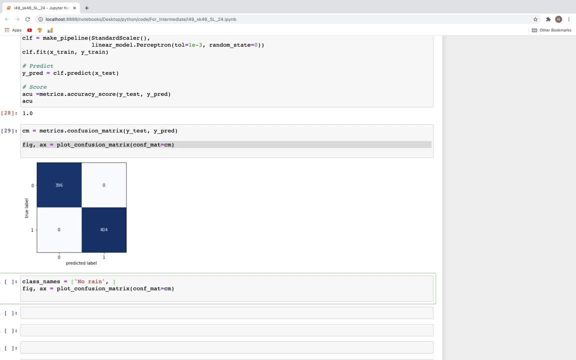 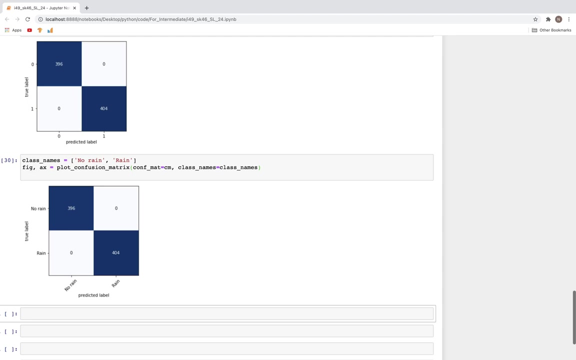 zero and one, and because we have class names, we can now specify a class names here is equal to class underscore names and when we run this, this is the confusion matrix that we get. so, for zero four are correctly predicted as kuin, so those with we running this, we go through the 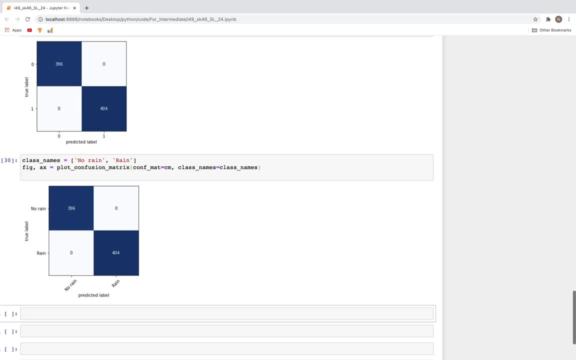 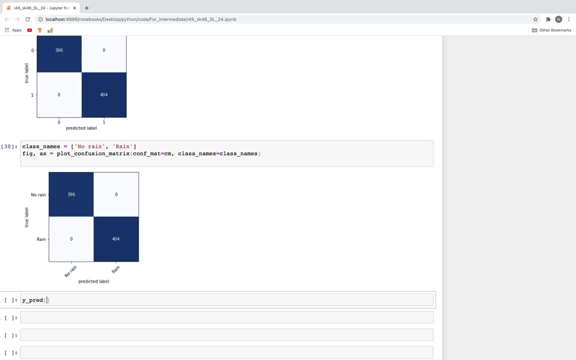 the images for clouds. and we can also double check that by looking at the sum of ones and zeros in the in the y pred. so y underscore pred is equal to one if you look at the sum of that and the one. so this is 404. so that's equal to what? 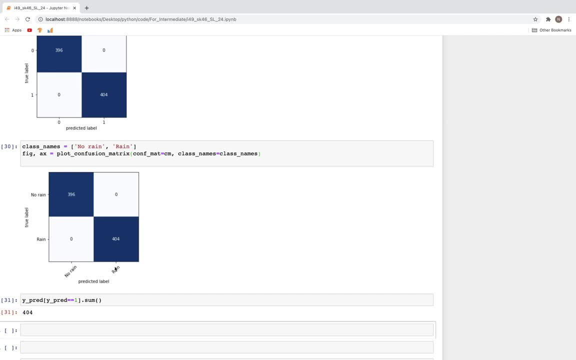 we have seen before, for the correct predictions of the cloud images as compared to the sun images. that was it for this video. i hope in this video you learned what is data augmentation and how it is used with the perceptron neural network or feed. one example of single layer neuron. 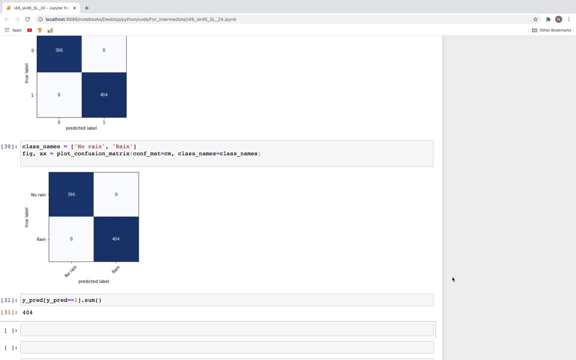 and, in the previous video, understood what data augmentation is. i hope you are able to apply this knowledge in a data set that you can create on your own and see what results you get. you can also try to apply this on the imaging, the mnist digits data set, using. 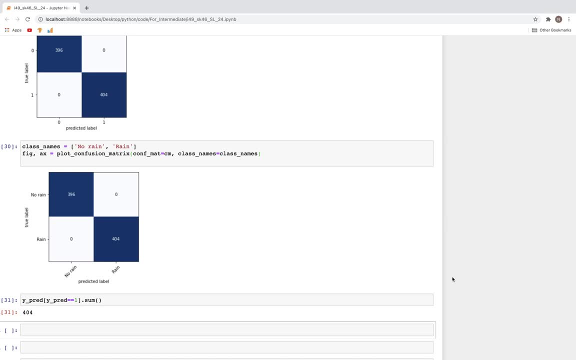 datasets: dot load underscore digits. i hope to see you all in the next video. please like and subscribe to my channel and i will see you in the next video. bye, bye, like, share and subscribe and if you have any comments, please let me in the comment section below. thank you.